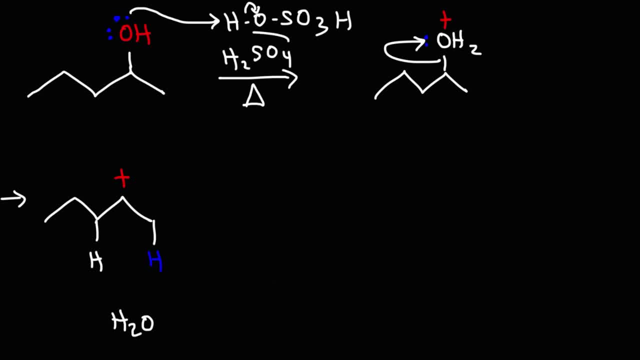 sometimes it could be bisulfate if you have a very, very concentrated solution of sulfuric acid. So water is going to abstract a proton and we're going to form a double bond. So that will lead to one possible answer. Now, water can also abstract the other proton adjacent to the carbocation. 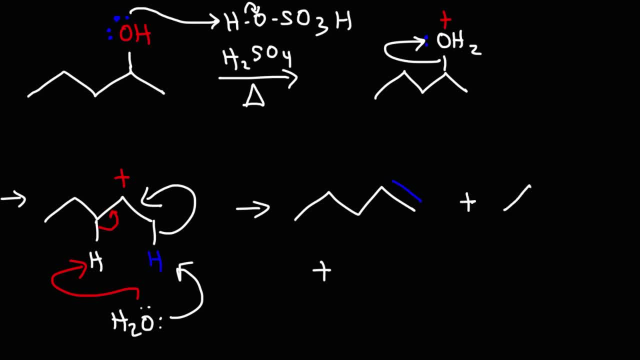 intermediate, giving us a different product, And so we can get either one pentene or two pentene, But two pentene is going to be the major product. This is the minor product. The major product is known as the Zates product. The minor product is the Hoffen. 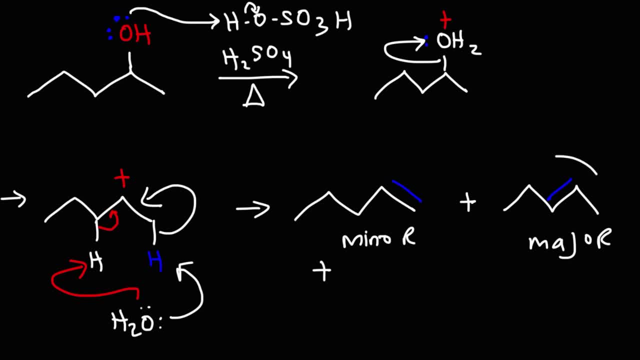 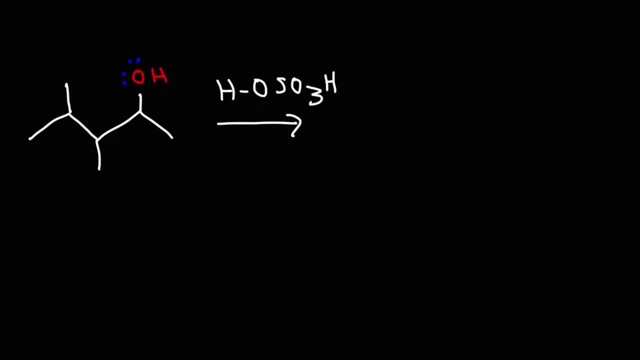 product. Now, keep in mind, you can get ofe the E isomer and the Z isomer, So just I want to mention that as well. Now let's work on another example. If you want to pause the video and work on this problem, feel free to do so. Go ahead and predict the major product of. 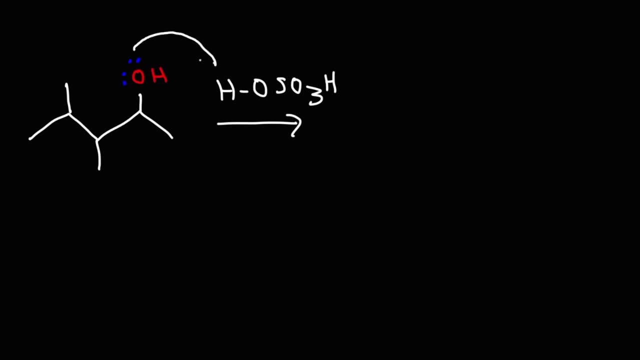 this reaction. So, like before, the first step is going to be protonation of the alcohol functional group. So there will always be two major products present in the mix. So in this example we have propсятone, suloku and tensyl weniger. 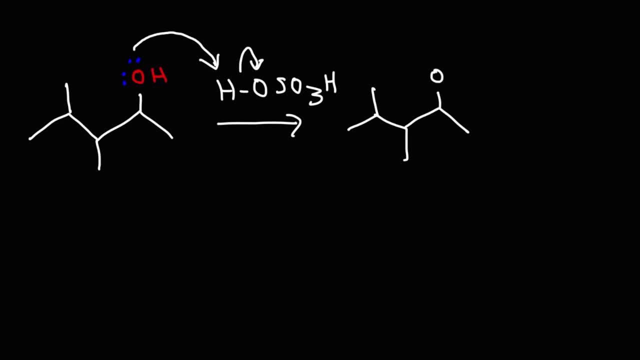 In the next step. the leaving group is going to leave Now. notice that we have a secondary carbocation intermediate. The plus charge is on a carbon that's attached to two other carbons, so that makes it a secondary carbocation, But that plus. 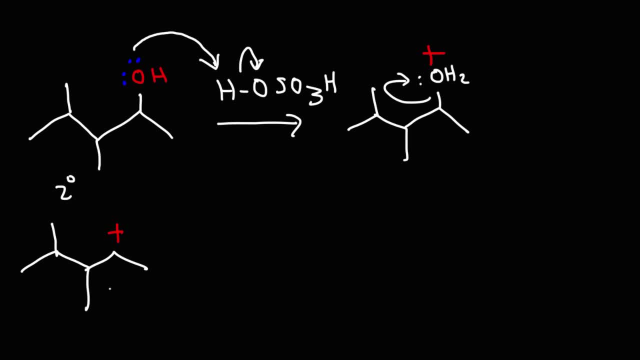 charge is adjacent to a tertiary carbon and when you see that a hydride shift will occur. Now the driving force for the hydride shift is carbocatine stability. A tertiary carbon, or rather a tertiary carbocatine, is more stable than a secondary carbocatine. so here's the 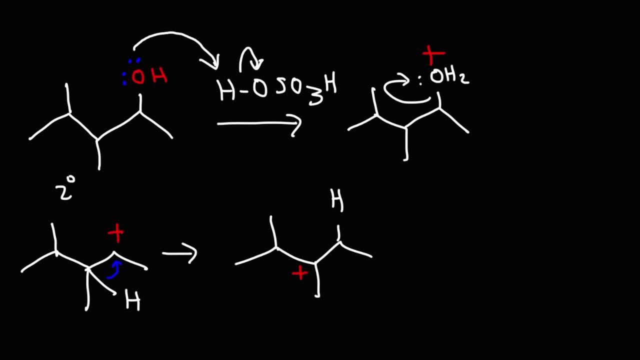 hydrogen now. So now, at this point, this tertiary carbocatine is going to determine a where we can get the double bond. So we can remove hydrogen one, a base can remove hydrogen two or it can abstract hydrogen three. So if the base abstracts proton three, 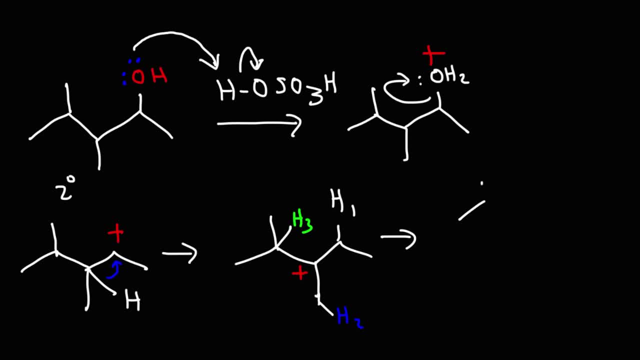 the double bond will form in this vicinity, giving us this product. Now let me put that in green: If the base abstracts proton two, we can get this product, And if the base abstracts proton one, we can get this product. 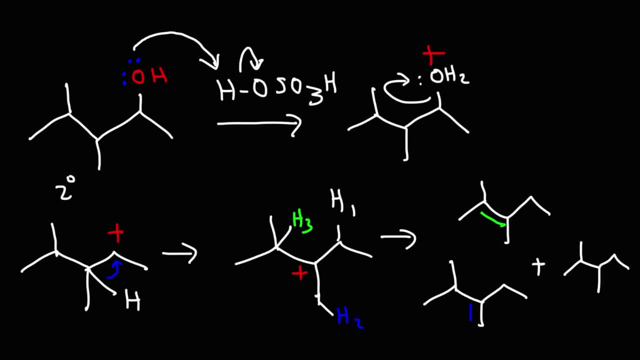 So which of these two products is the double bond? So which of these three alkenes is the major product? What would you say? A double bond with four R groups is going to be a more stable alkene than one with three R groups. 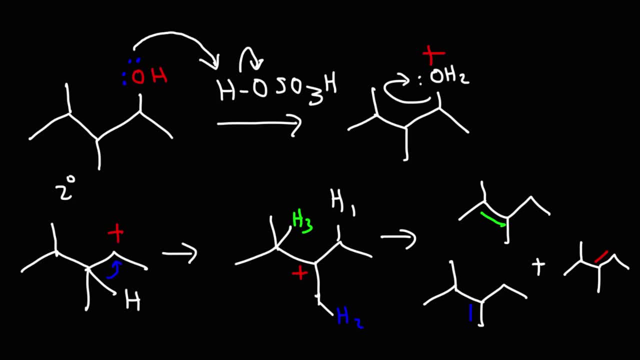 and that's going to be more stable than one with two R groups. So if we look at the double bond highlighted in blue and we focus on the two carbon atoms that are part of the double bond, how many other carbon atoms are attached to those two? 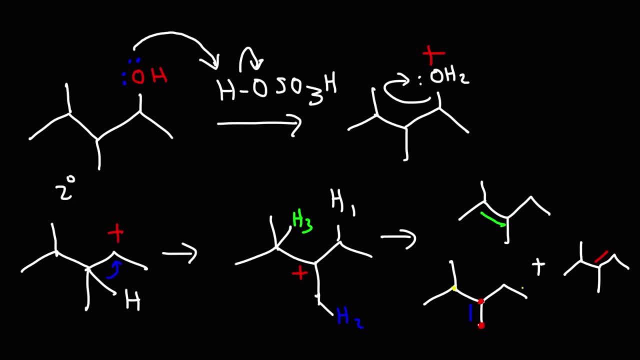 double bonded carbon atoms. For this one there's only two, so it has two R groups. For this one here on the right, these are the two double bonded carbon atoms and there's three other carbon atoms attached to it, so it has three R groups. 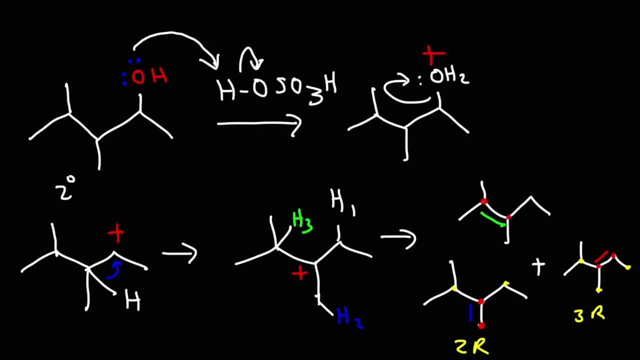 And for this one there's four carbon atoms that are attached to the two double bonded carbon atoms, so it has four R groups. So this is what is known as a tetrasubstituted alkene. It's going to be the major product. 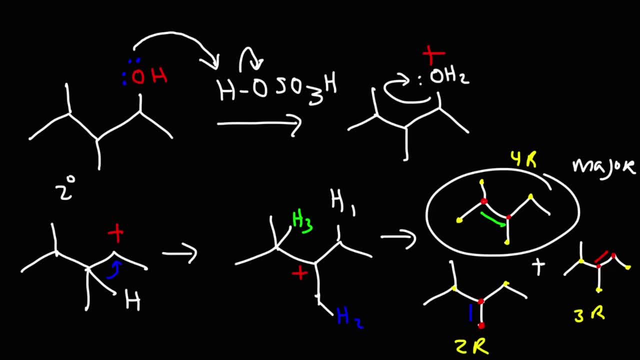 because it's the most stable alkene that we can form. So remember when taking a test and when you're dealing with an E1 acid-catalyzed dehydration reaction of alcohols with like sulfuric acid, the major product is typically 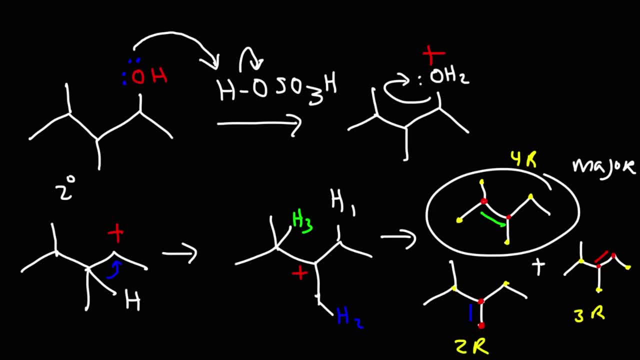 the most stable alkene product that can be formed in this reaction. So you want to look for the alkene that's highly substituted, particularly an internal alkene as opposed to a terminal alkene. Now, from this point forward, we're just going to focus on 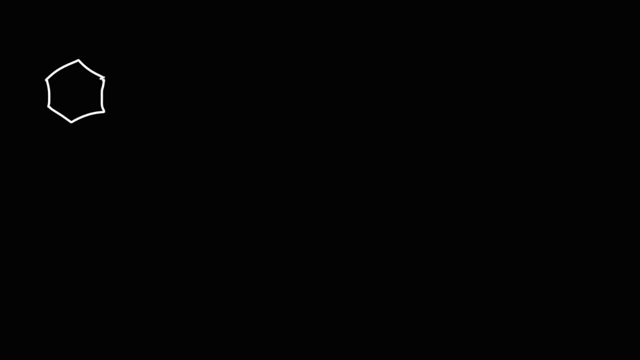 drawing the major product and writing the mechanism to get there. So feel free to work on this example. So, as always, step one is protonation, Step two is the leaving process, So the carbon group leaves. So right now we have a secondary. 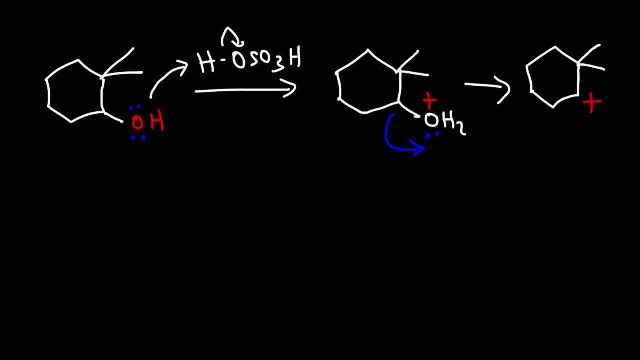 carbocadine intermediate. Now note that the carbocadine is adjacent to a quaternary carbon with two methyl groups attached to it. So what's going to happen is, instead of getting a hydride shift, we're going to get a methyl shift. 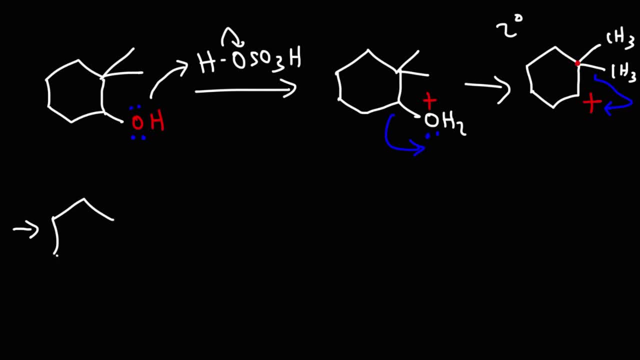 So the actual carbon structure will change Now because the methyl moved towards this carbon. that carbon no longer has a positive charge, But the carbon that lost the methyl group it now carries a positive charge. So we went from a secondary carbocadine. 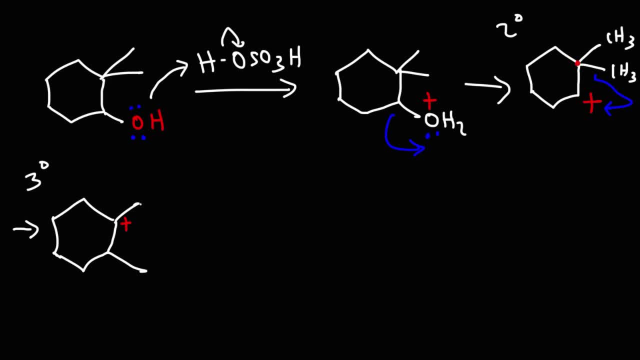 to a tertiary carbocadine. So now at this point we can get the different products in this reaction relative to the carbocadine. So we can abstract proton one and form a double bond here, or we can abstract proton two and form a double bond here. 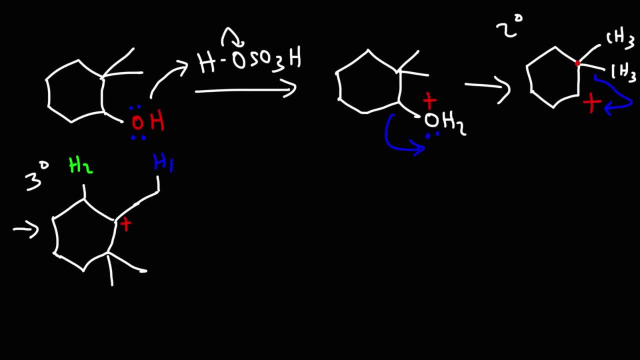 or we can abstract proton three, giving us a double bond here. Which proton will lead to the most stable alkene? If we put a double bond here, this will be a disubstituted alkene. If we were to put a double bond here, 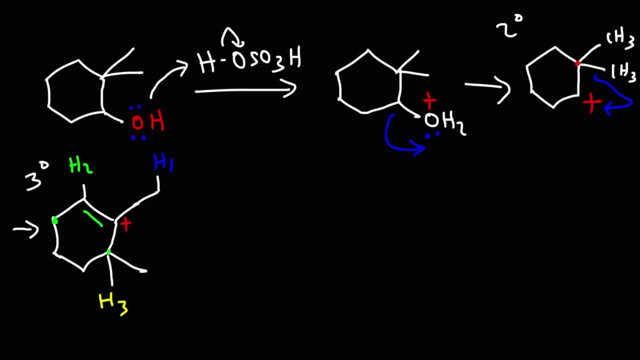 this would be a trisubstituted alkene, And if we were to put a double bond here, this would be a tetrasubstituted alkene. So therefore, the base will preferentially abstract proton three, Because by doing so, 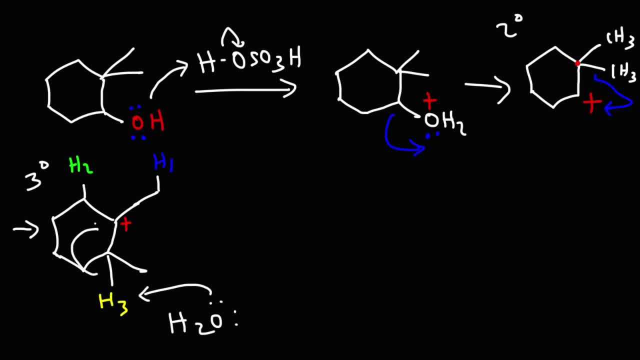 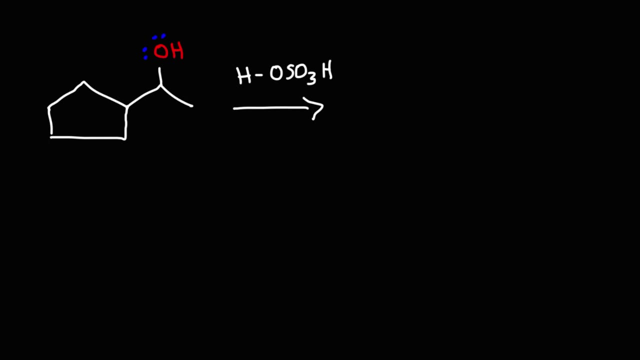 we're going to get the most stable alkene in this reaction. So this is going to be the final product, the final major product, of this reaction. Now let's work on this example. So here we have an OH group attached to a carbon structure. 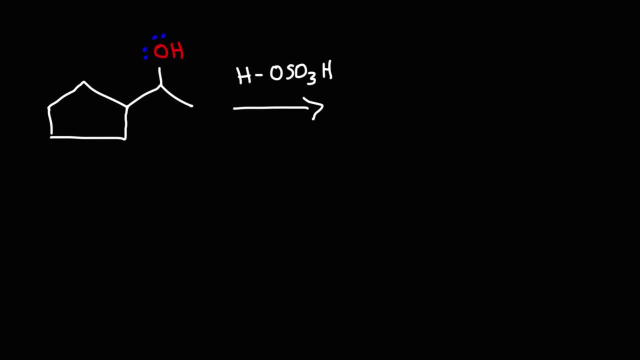 that contains a ring. When you see this, you need to watch out for ring expansions. So, as always, the first step is protonation, followed by the escape of the leaving group. When the leaving group leaves, we're going to get a secondary. 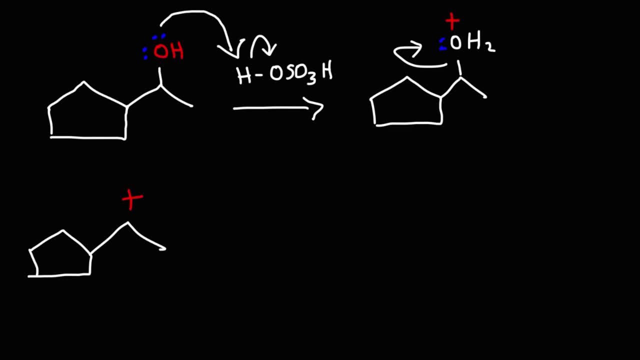 carbocation intermediate. Now let's see what's going to happen here. because this secondary carbocation intermediate is adjacent to a tertiary carbon, So a hydride shift can occur. If the hydride shift occurs, the plus charge will move here. 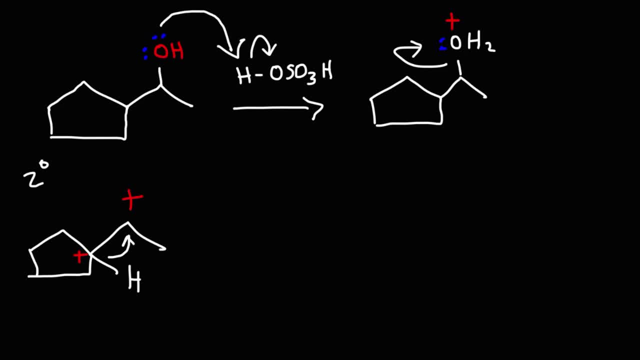 And we'll simply have a five carbon ring with a tertiary carbocation. However, that's not the most stable rearrangement that we can make, Because the ring can expand and still yield a tertiary carbon. A six carbon ring is more stable than a five carbon ring. 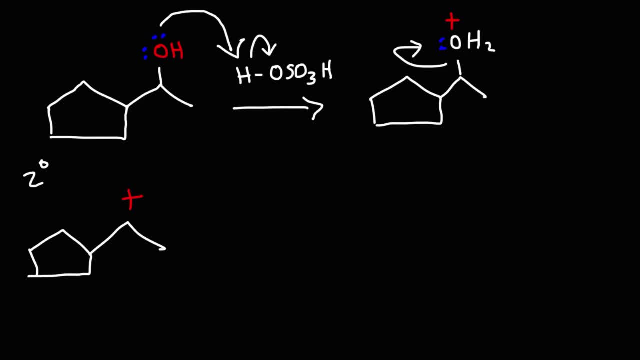 Thus, stability is the driving force for carbocation rearrangements. A carbocation will rearrange to find the most stable configuration possible. Now let's number these carbons accordingly. The bond between carbons two and six will break and the electrons in that bond 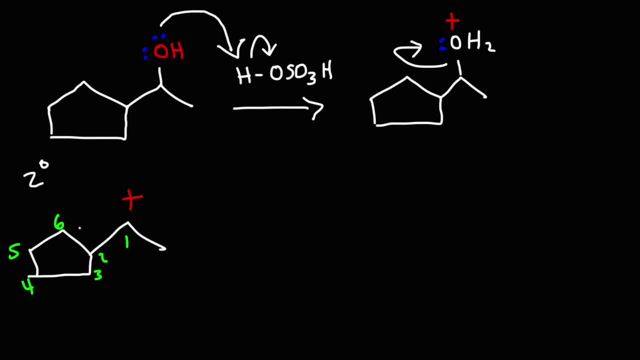 will be used to break the carbon. Now, the bond between carbon two and six will be used to connect carbon one and carbon six. Thus, the structure that we're going to obtain will look like this. So this is carbon one. This is going to be. 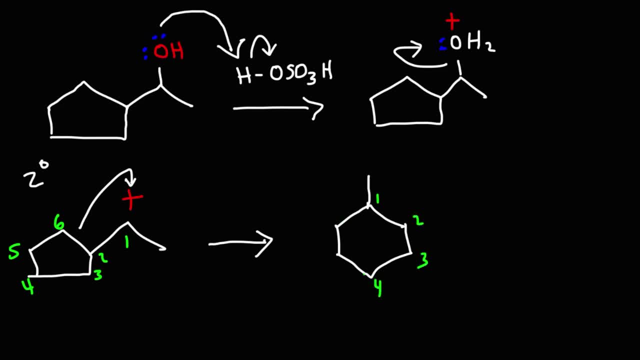 carbon two, three, four, five and six. So six is now attached to carbon one and we still have the methyl group attached to carbon one. The question is, where is the positive charge? Carbon two and six lost the bond. 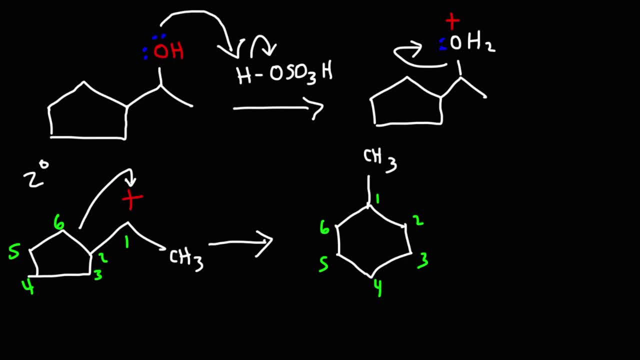 and one and six. there was a bond that formed between those two, So two lost the bond but didn't regenerate it. Therefore the plus charge is on carbon two Now. right now we have a secondary carbocation, but a hydride shift will occur. 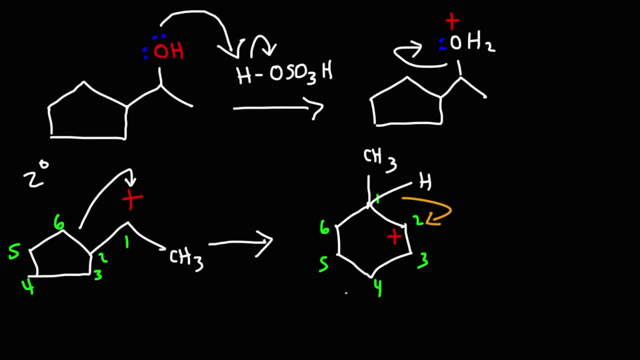 to give us a more stable tertiary carbocation. So after the hydride shift, the plus charge is now on a tertiary carbocation, which means we could form a double bond here, here or here. This will give us a di-substituted alkene. 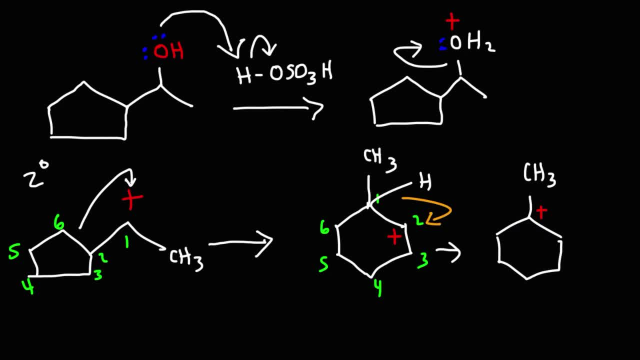 and putting it here or here doesn't matter, So we can just pick one of them because of the symmetry. So the base is going to abstract a proton form, a pi bond, and that's it So the final product that we're going to get. 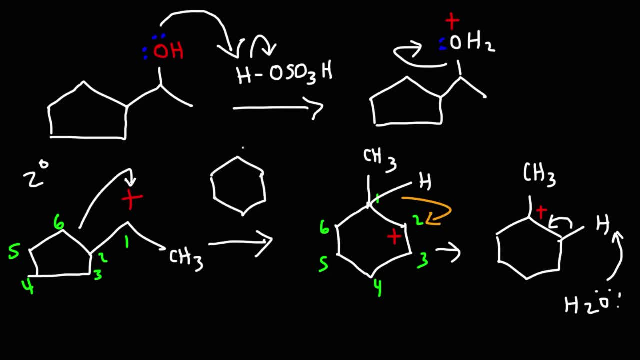 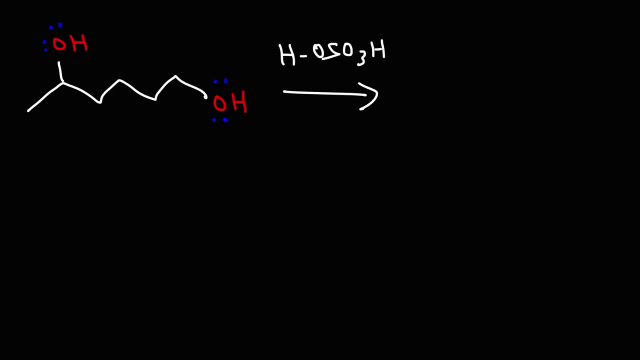 let's see if I can fit it here- is going to look like this. So that's the major product of this reaction. Now let's work on this example where we have a molecule with two alcohol functional groups. So what's going to happen in this reaction? 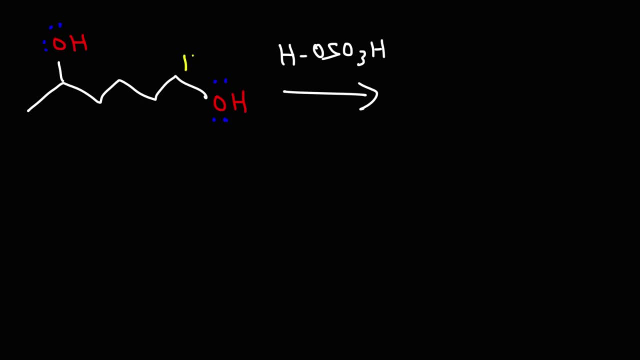 So we have a primary alcohol and we have a secondary alcohol. Which one will be protonated? The fact is, both can be protonated, but the mechanism by which the reaction will work will be adjusted. So let's focus on protonating the secondary alcohol first. 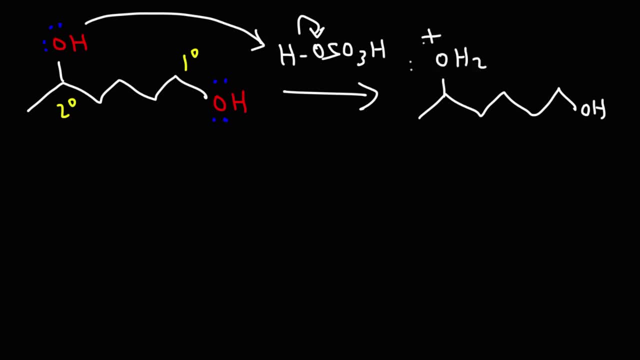 So it's going to become a good leaving group and when it leaves it's going to leave behind a secondary carbocatine. Now, at this point we could form an alkene if we abstract a nearby proton, but the oxygen 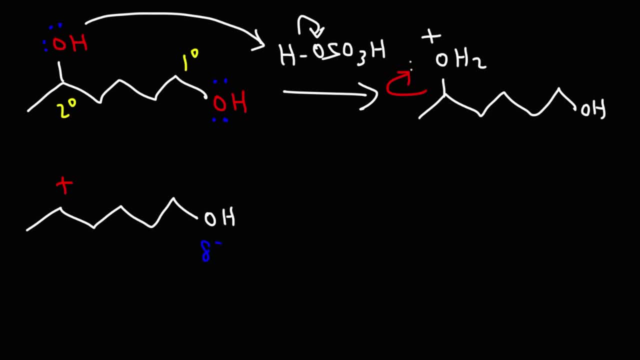 it's going to be attracted to the positively charged carbocatine, because oxygen has a partial negative charge And that electrostatic attraction is going to pull the oxygen towards that carbocatine And that's where we're going to get an intramolecular reaction. 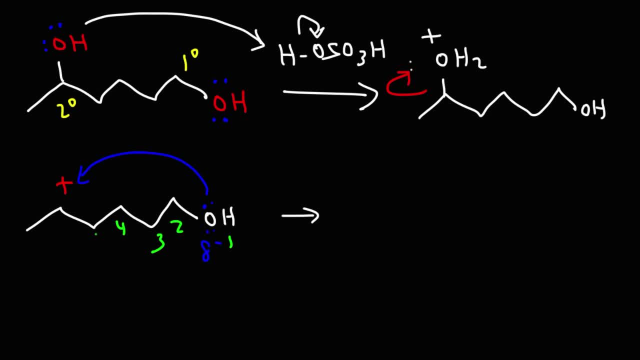 Let's call this one, two, three, four, five, six. So we're going to get a six-membered ring with oxygen being part of that ring. This is going to be number one, two, three, four, five. 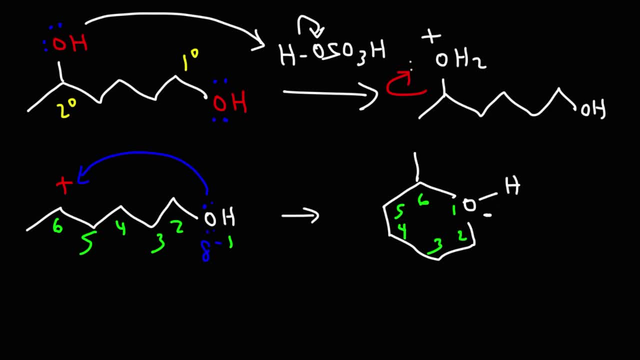 and six, So we still have the methyl group on six, and the last thing we need to do is remove the hydrogen on the oxygen, And so we could use water to do that. Thus, for this particular reaction, instead of getting an elimination reaction, 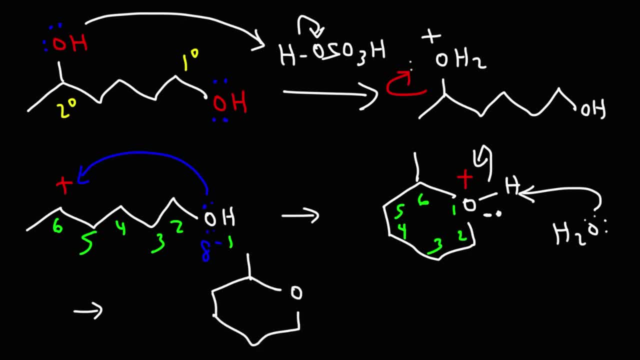 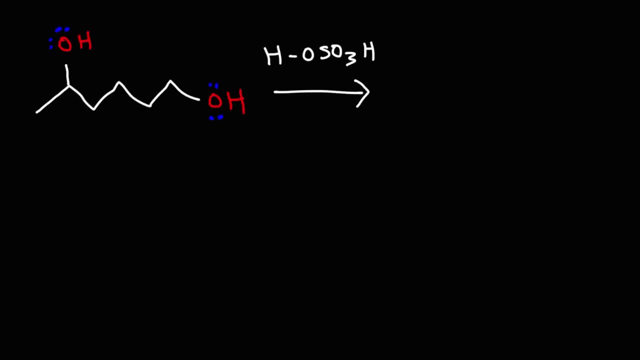 we can get a cyclic ether. So this is more of an SN1 reaction. The leaving group leaves, we get a secondary carbocatine and then the nucleophile attacks, the secondary carbocatine giving us the product. Now let's focus on protonating. 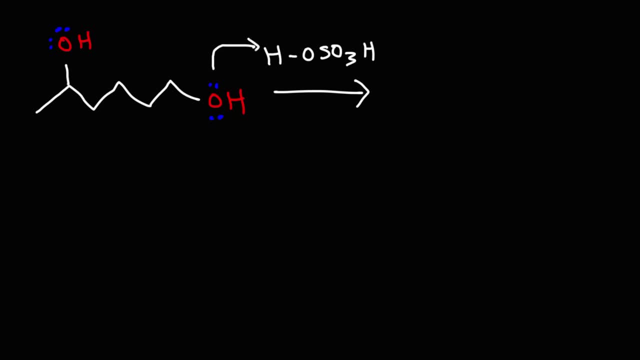 the primary alcohol as opposed to the secondary alcohol, And let's see how the mechanism is going to change Now. the leaving group won't just leave on its own, because if it does so, it's going to leave behind an unstable primary carbocatine. 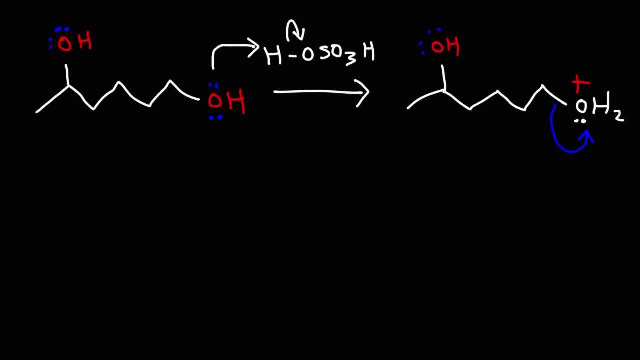 It's going to leave behind an unstable primary carbocatine intermediate. Primary substrates don't favor an SN1 reaction, So this is not going to it's not going to be the most likely scenario to occur. Instead, the oxygen will act as a nucleophile. 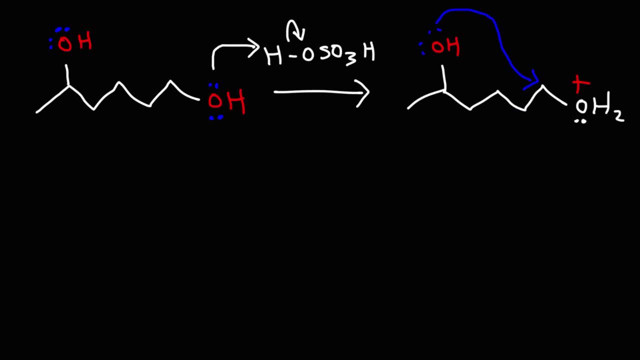 and attack the primary carbon, which is highly accessible, kicking out the leaving group, And so this reaction resembles an intramolecular SN2 reaction. This is going to be carbon one, two, three, four, five, six, So we're still going to get. 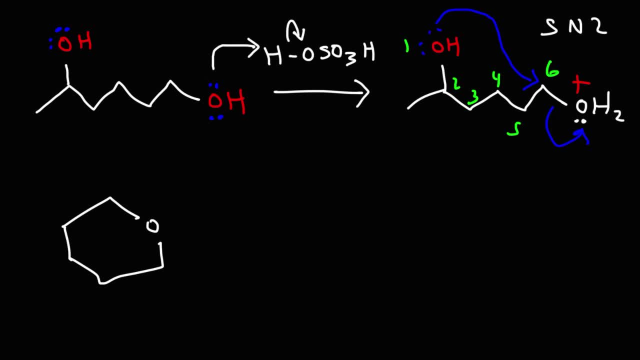 a cyclic ether, but it's going to look a little different, So let's call this one, Let's call this, or I guess we can call this two if we just count it the other way. In actuality it looks the same.